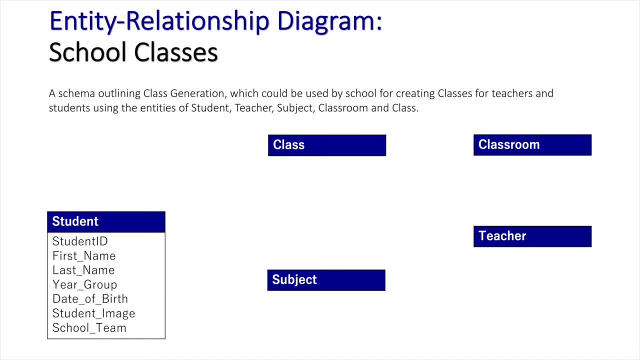 mapped to data on the database and it's actually the student ID that's on that card. that helps reference all that data about the student. Next we'll look at class, and this is all the information about each class in the school. Okay, so we're going to put. 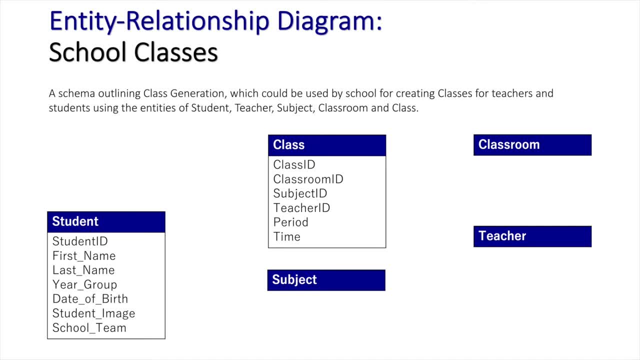 them together and these are the things we need to have to make a class. Okay, every class has a specific code. They all have a classroom, They're all based on a subject, They all have teachers. Okay, they'll have a specific period and a specific time. Okay, and you may notice students not sitting. 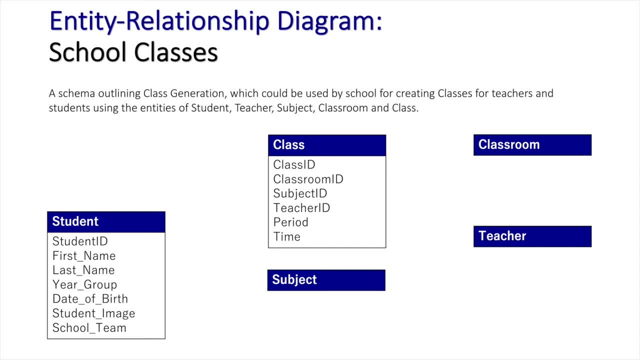 in there at the moment, Okay, and we'll explain that as we get to the relationships in this video. The next area to look at is subject: Okay, and with subject, each subject has a specific code, Okay, and they all have specific requirements, Okay, which they may require to be in a specific room. 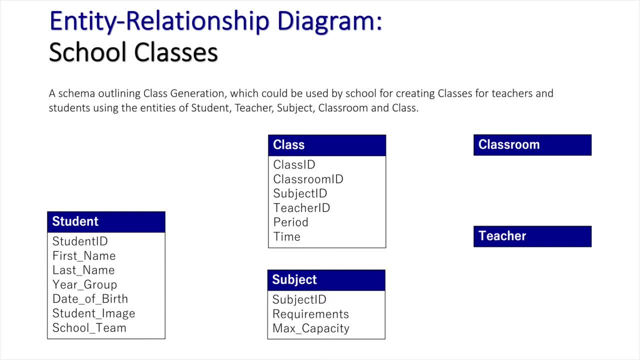 and a max capacity Students that can do the subject. Usually it's around 30 students in most mainstream subjects, but technology-based subjects sometimes have a capacity of 25 students as their max capacity due to safety reasons. So that needs to be factored into our database because then when making classes, 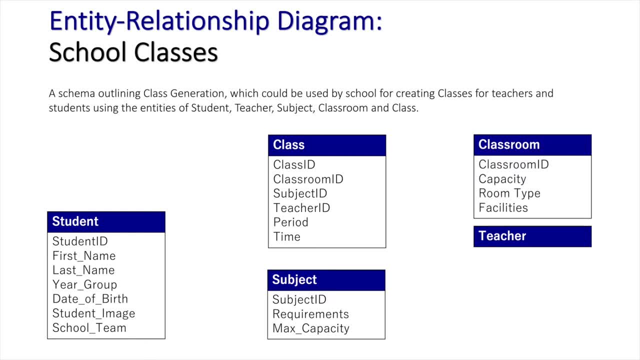 we can't have more than 25 students in them Going on. next we have the classroom, and every room obviously has a number and that's based will be the basis for the classroom ID. Every room has a specific capacity of students that can fit into that room. Okay, which correlates with what we're 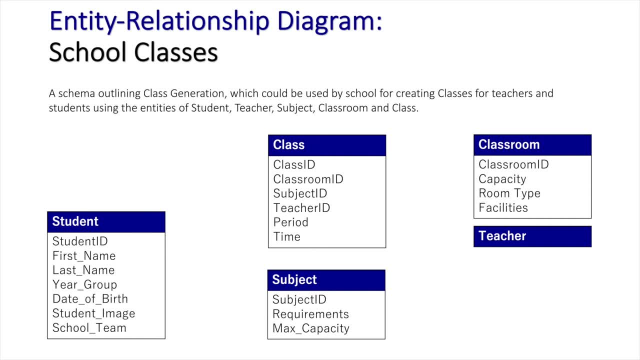 saying about each subject. We can't put 30 students into a room with only 25 seats, so that needs to be recognized, as well as the room type. We might be in a kitchen for hospitality. We may be in a wood tech room. Okay, we may be in a science lab. 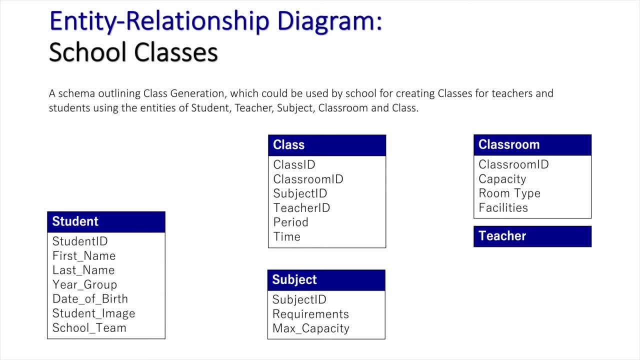 and obviously that really needs to link to the subject being done in that room. And then finally is facilities, so they could be obviously managed and the right subjects go to the right room for specific classes. The final area is teacher. Every class obviously needs a teacher teaching students. 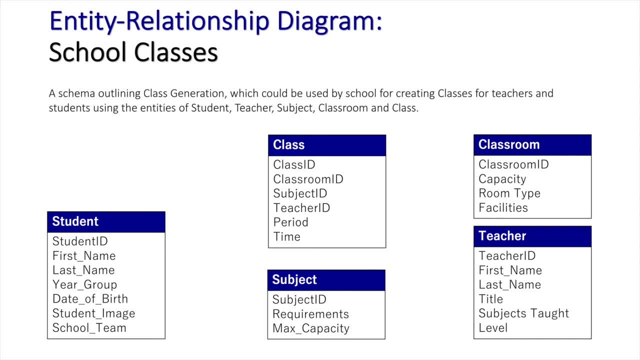 what to do. Okay, and teachers, just like students, have their own ID. It's usually based on their first name and last name being combined together, but that all depends on how the database has been created, and that is, does record data about teachers, such as their first name. 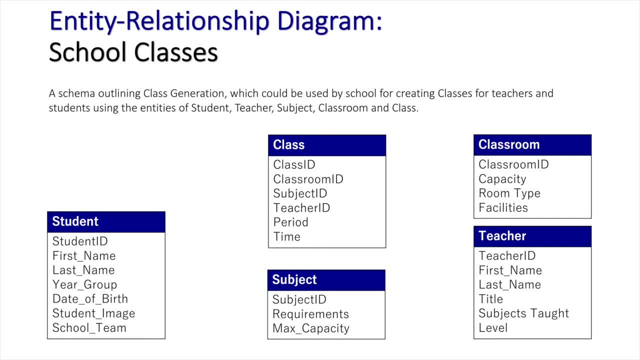 their last name, their title- Okay, which might be, if they are actually a Mr or Mrs- the subjects they teach and then, finally, their level: Okay, obviously we have classroom teachers, but then we also have subject coordinators, year coordinators, assistant principals- Okay, a whole variety of titles, Okay. 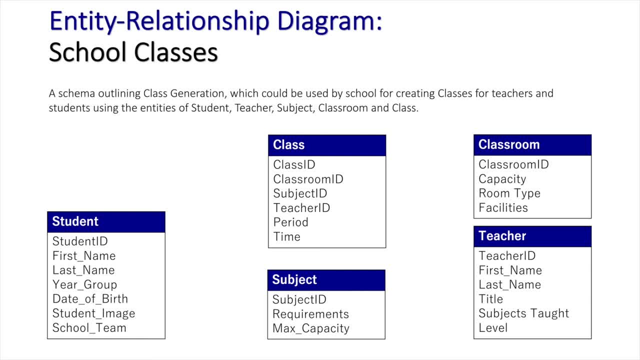 that needs to be mapped to the teacher and the database as well. So that is all the attributes that are going to be involved in the entities we're using in this relational database. What we've now going to do is establish our relationships, connecting all the data together, And we're going 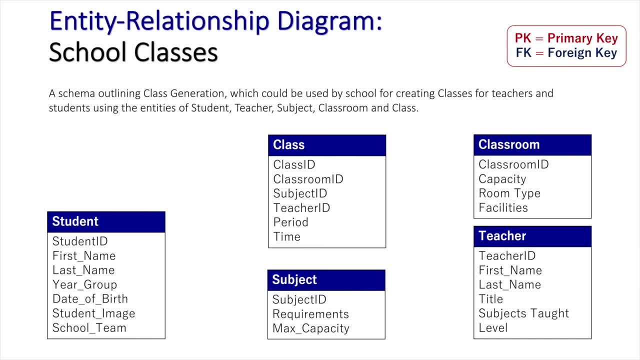 to create these relationships, as always by connecting our primary and foreign keys. And if you know your primary and foreign keys, you can already probably see where a lot of these relationships are going. So firstly, look at classroom. One class only has one classroom, but a classroom can be used. 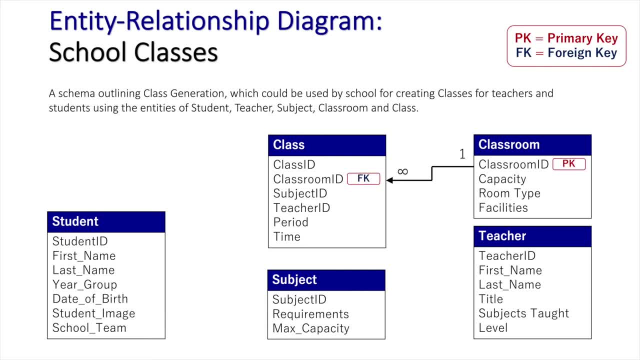 for multiple classes, so that is going to be a one-to-many relationship. The same thing goes for a teacher. Okay, has one teacher, but a teacher can teach multiple classes. so once again, a one-to-many relationship. you can see that primary key connecting to its foreign key in class and subject is exactly the 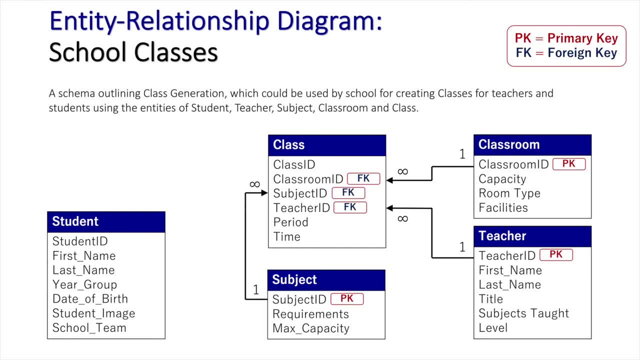 same. every class is only based on one subject, but there might be multiple classes for a specific subject. so once again, another one-to-many relationship. the only one that really differs here is student. okay, because there are multiple students in multiple classes, making it a many-to-. 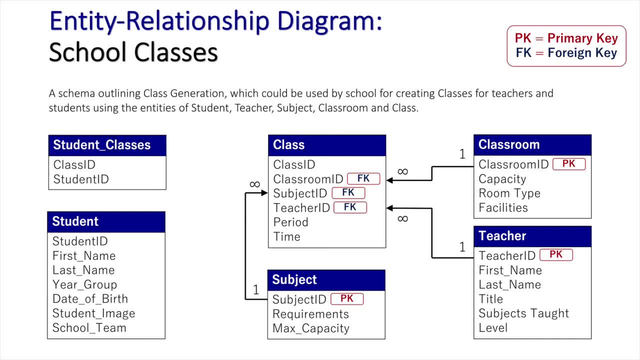 junction using both primary keys in the actual junction. so that means we can actually reference one student to multiple classes and we can re-reference a class to multiple students. so I hope that helps you understand the use of the junction here for establishing the many-to-many relationship between student and class and why we don't have a student foreign key sitting there in. 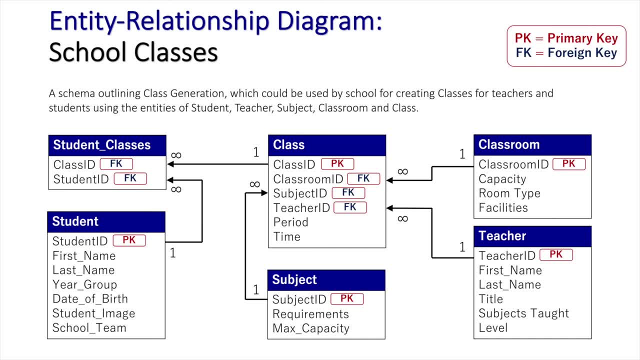 class because we actually have to use the junction so that both have their individual records, being able to reference multiple records in the actual junction, The corresponding entity. so I hope this gives you an overview of how I believe a school database relational database may work okay and really a lot of them are one-to-many relationships because 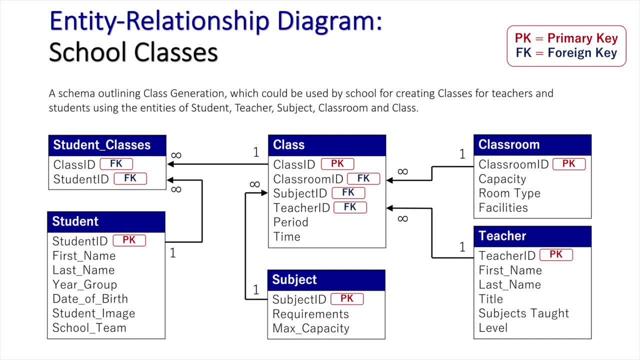 we only have one classroom, one teacher in one subject being taught in every individual class, but there are multiple students in a class, in multiple classes, which is a many-to-many relationship, and thus we have to use a junction.